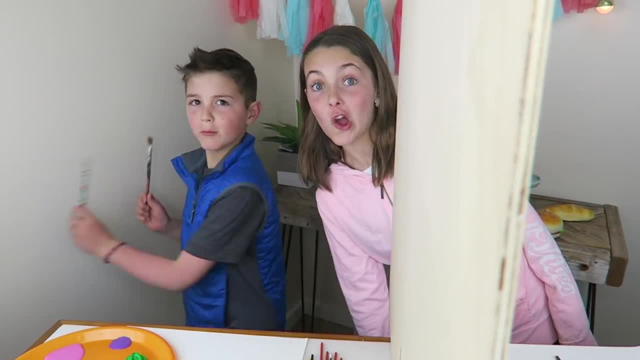 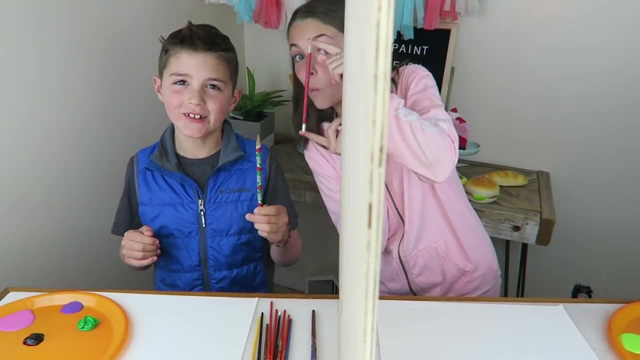 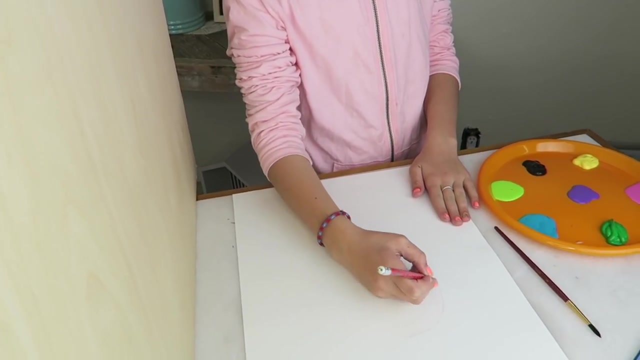 surprises to each other at the end. Okay, let's get started. So first I'm going to be using my pencil So I can trace it out, and then start painting. So I'm just going to draw the outline of Axel's head. 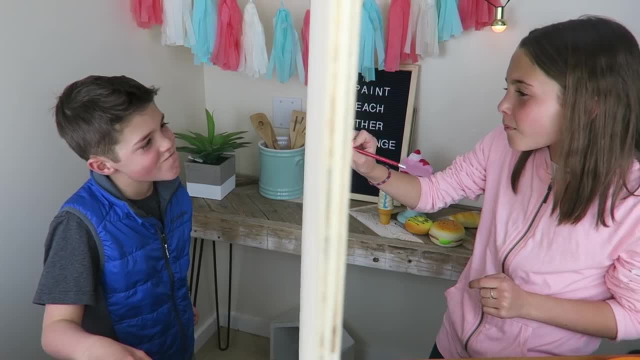 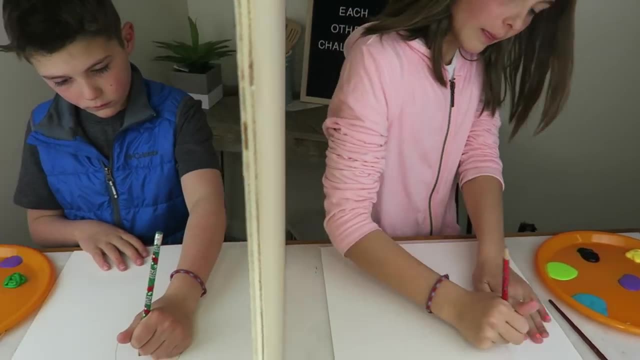 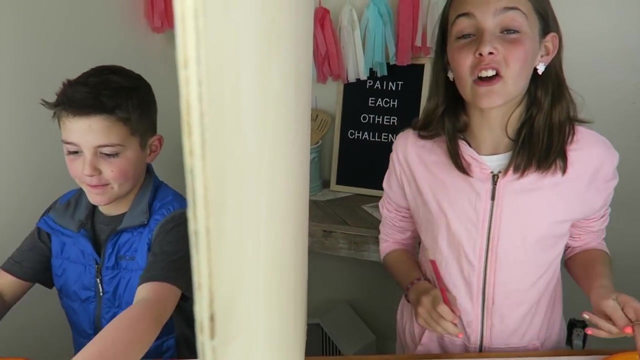 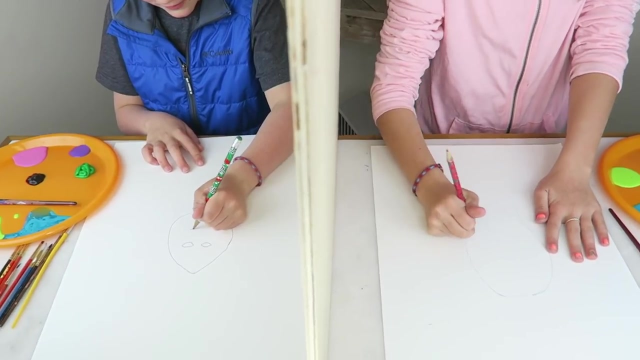 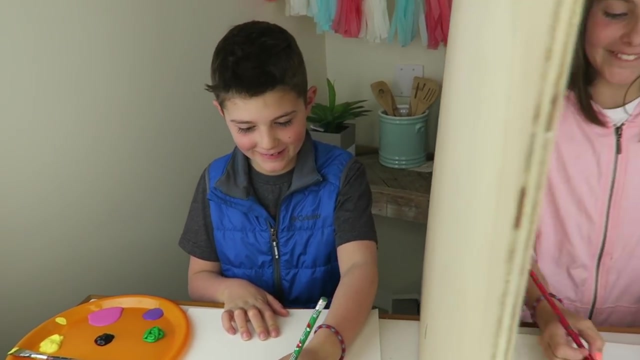 Axel, look at me. Okay, I kind of have an advantage because I've been in art class longer than Axel and I'm kind of older, so I'm going to paint his head If I'm gonna make you happy. Okay, guys, I don't want Axel to know, so just look. 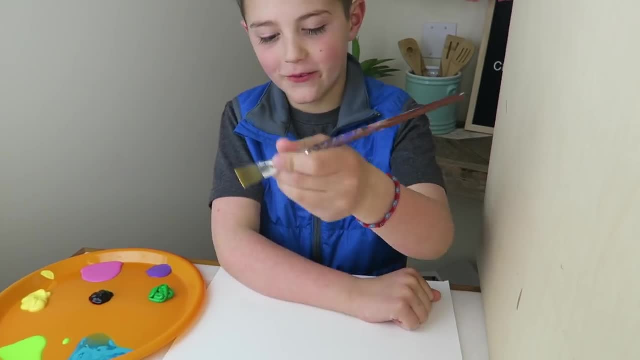 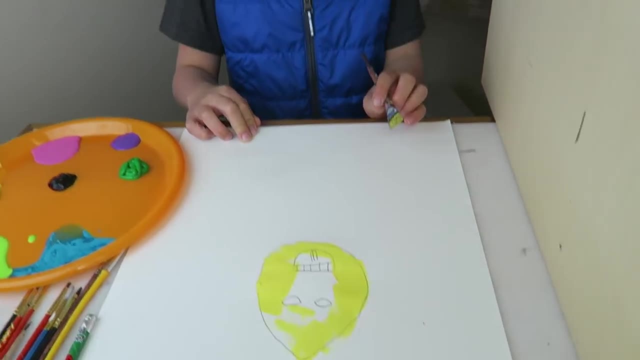 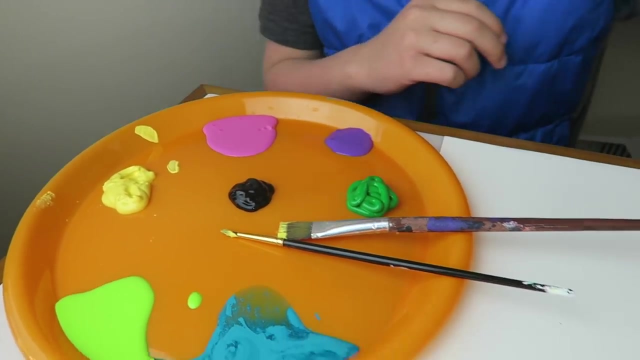 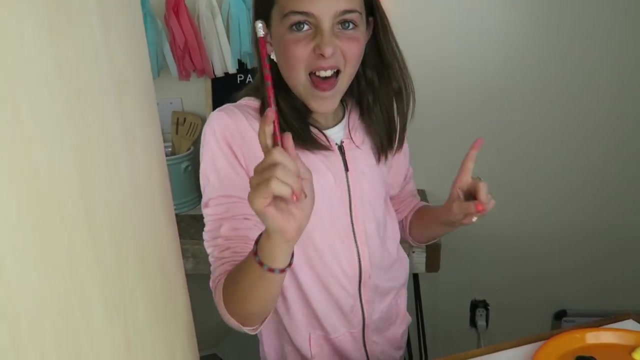 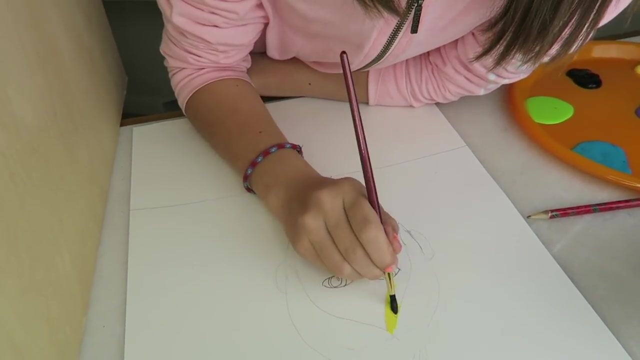 All right, guys, I'm ready for my paint. I'm going for yellow. It kind of looks like it. It looks like a weird eyed alien. I'm sorry, I'm sorry. There we go. First stroke of paint, Ava, let me see your eyes- Greenish. 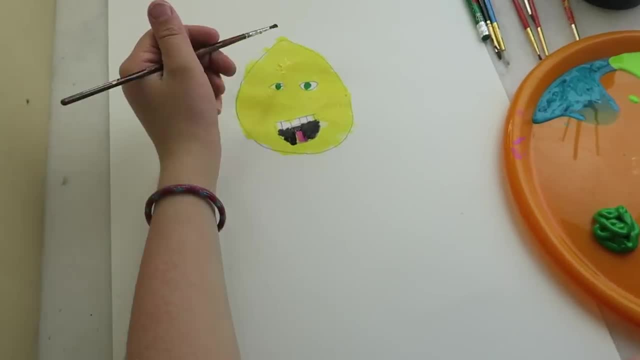 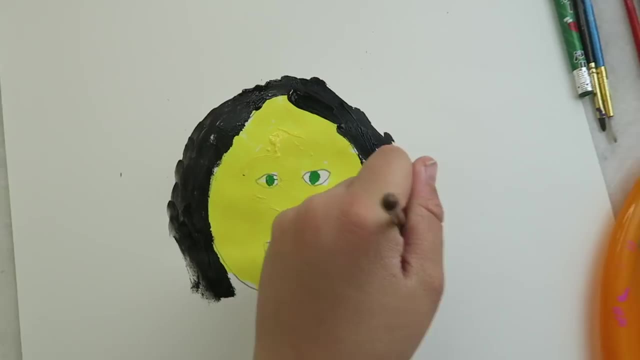 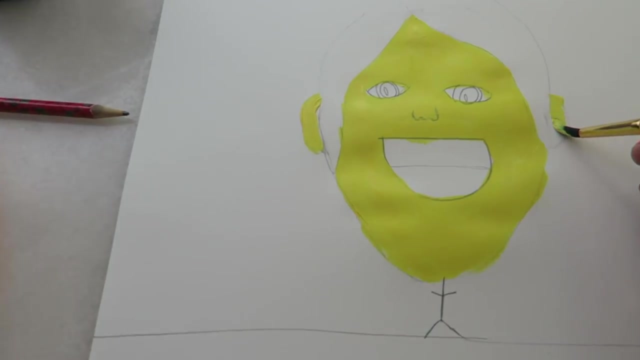 It's an egg Green. All right, All right guys. right like that. It's going to look like willow. What hold will it look like It's a mead. What am I putting down here? A beaded. 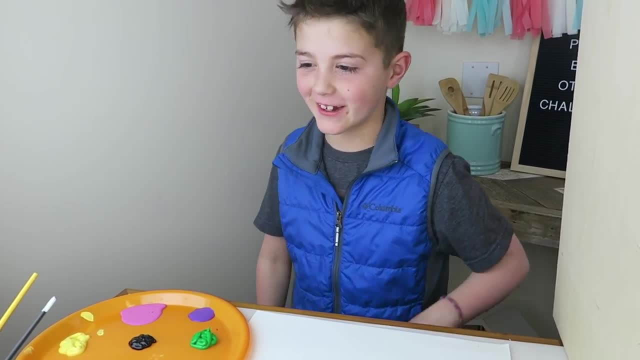 cules. What kind of headset was Axel wearing in class? A beaded mask. What is that? Peppymothers, Earthworms, A watermelon, Spider, myses. What is that? A snot, A seagull. 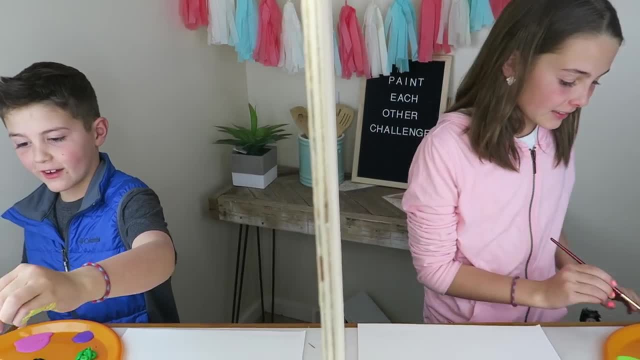 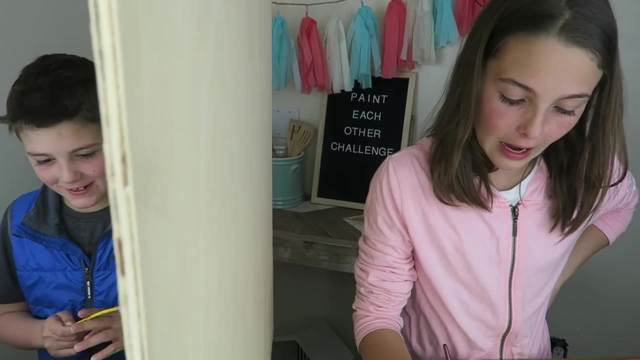 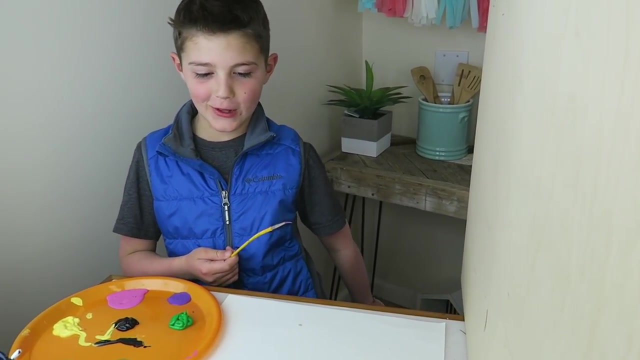 Yeah, If I wanted to eat them, because they barely have anything on them, or you want to eat that brown, I'm gonna make your hair black. all right, even how you looking, it's looking like Elvis. how's yours coming over there? well, it's kind of looking like a yellow blob. it's kind of plain. so I'm gonna add. 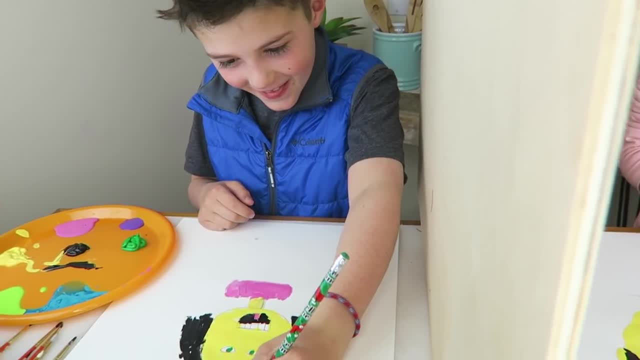 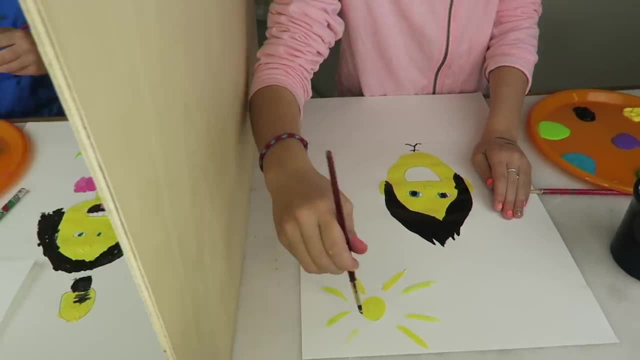 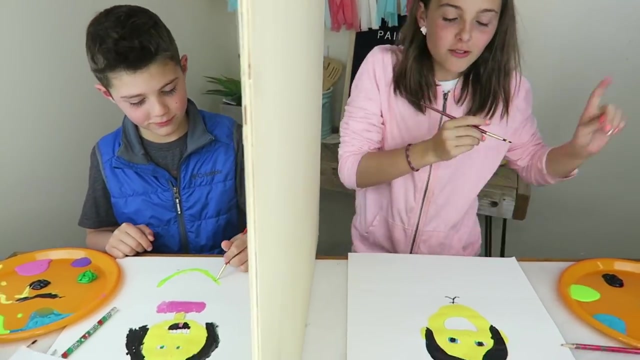 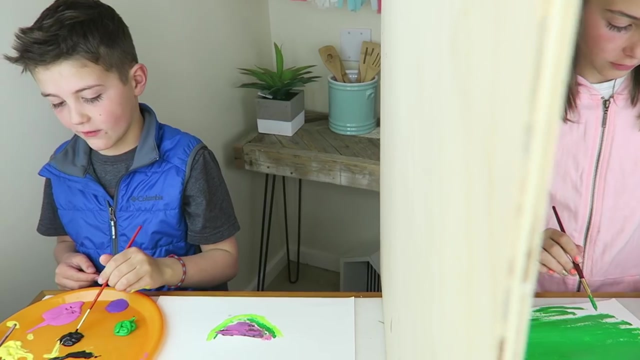 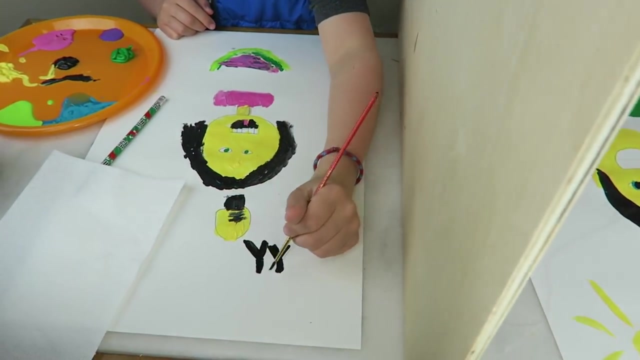 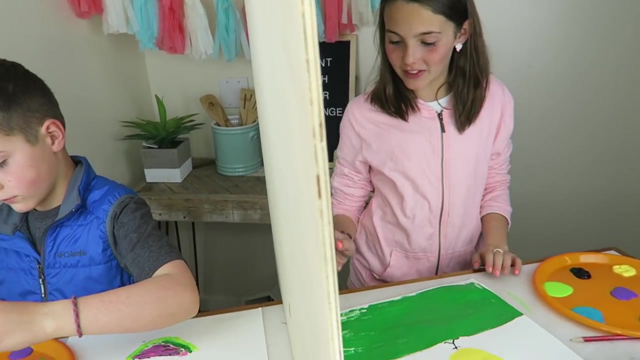 something. oh, I know I'm gonna do. hey, just, you know, this is you in the summertime. same, this is you in the summertime too. thank you, wait, Braxel, to see my little masterpiece. I will be your beautiful servant. It'll be like he's looking in a mirror. 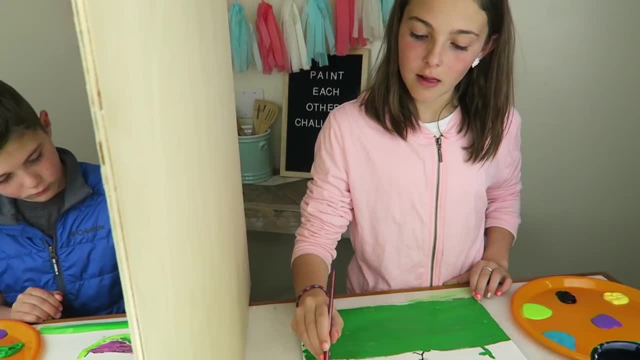 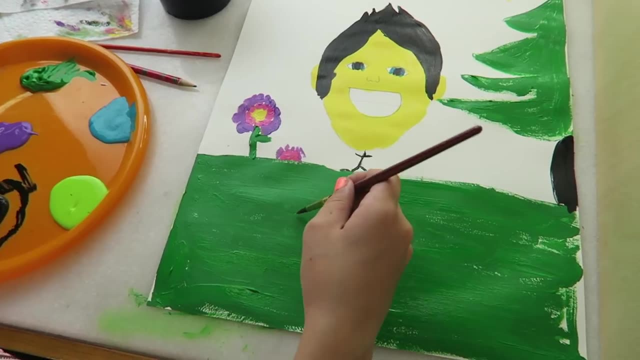 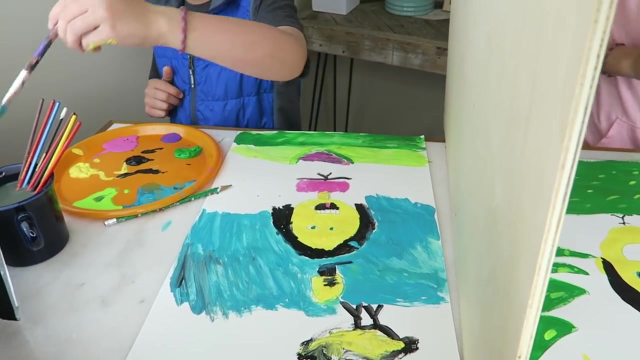 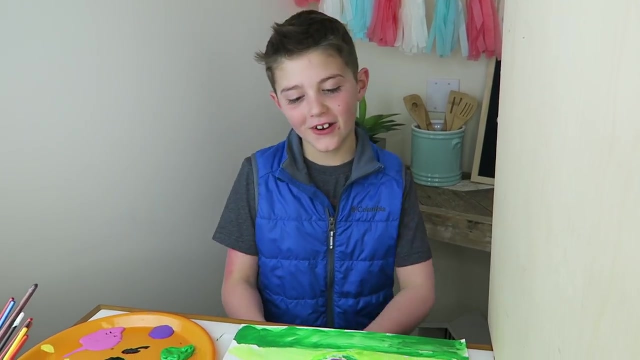 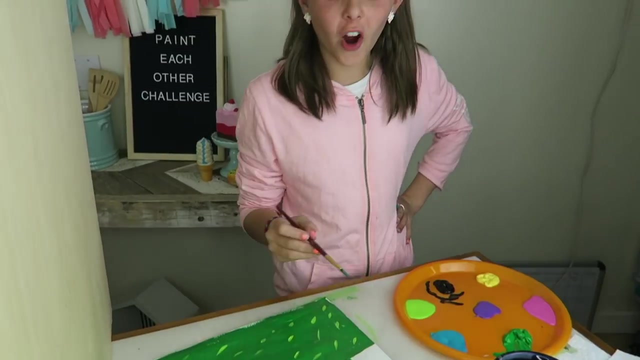 Going to draw a pretty tree in the background. Just gotta fill in those white spaces And I'm done. I feel like it needs something more. So the hardest part was Ava's eyes, mouth and all of her. The hardest part about this picture of Axel. 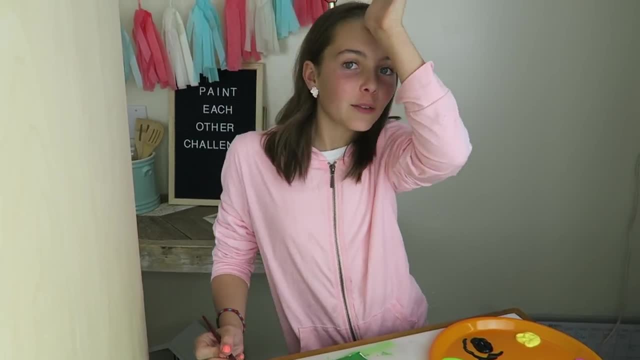 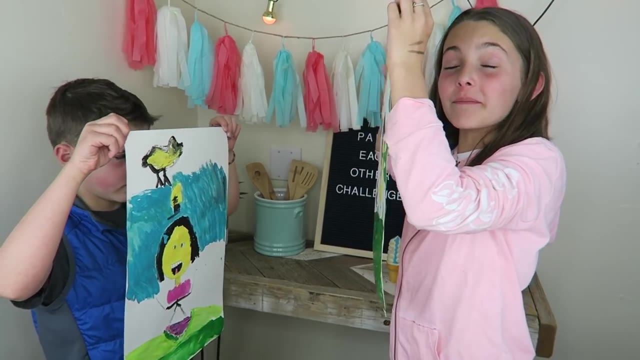 was probably the hair Cause he has like this weird wavy hair that's up in a spike. What are you talking about? On the count of three, me and Axel are going to show each other our pictures. One, two, three. 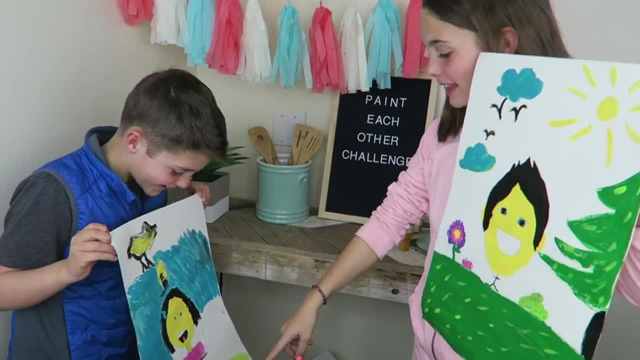 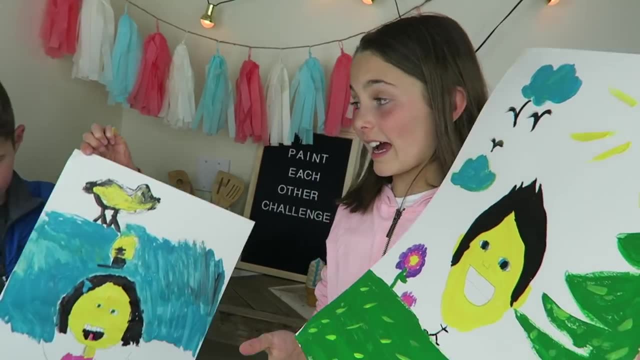 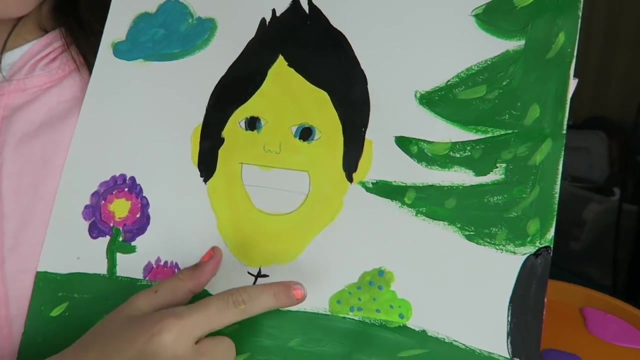 Whoa, Is that a watermelon? Uh huh, Whoa, Is that a blueberry bush? Yep, Okay, guys. so Axel has a lot of detail in his. We got his blue eyes, the blueberry bush. a flower, some grass. 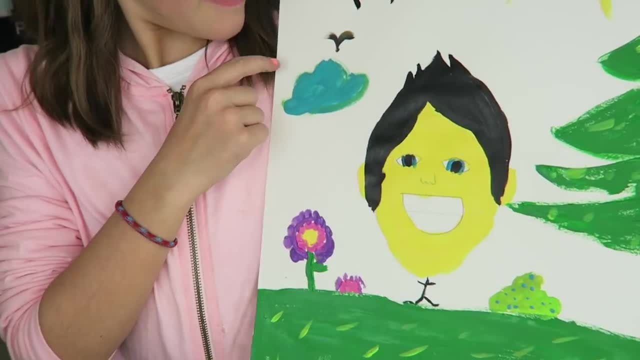 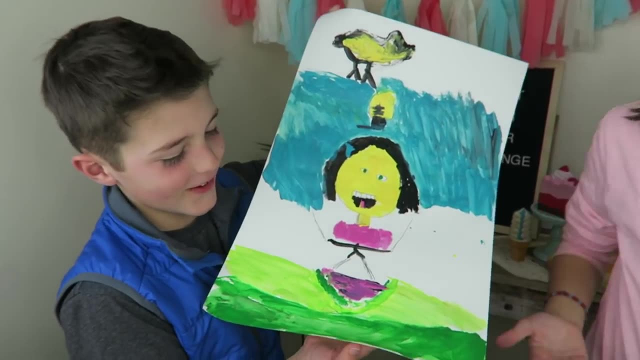 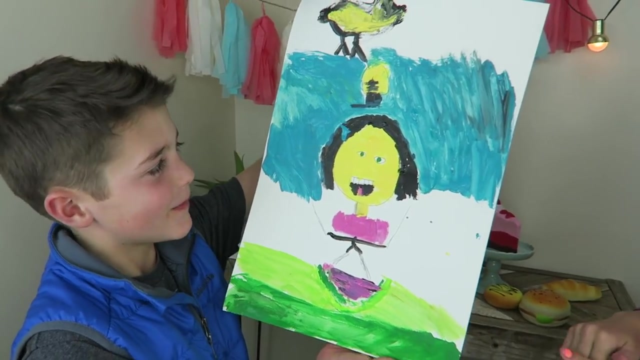 Some tiny bodies: A tree- yeah, tiny body- A cloud and a few birds And, of course, the sunshine Ding. So Ava has. she has a chicken flying above her, She has a light bulb above her head. for an idea. 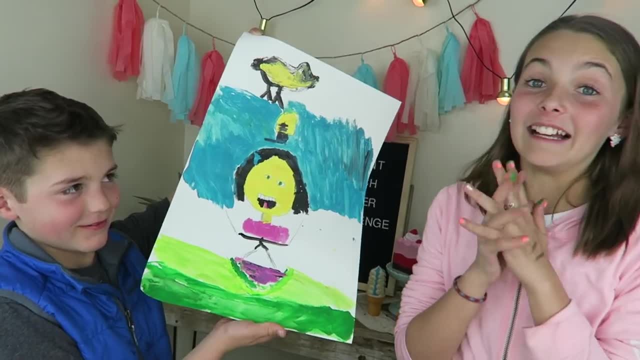 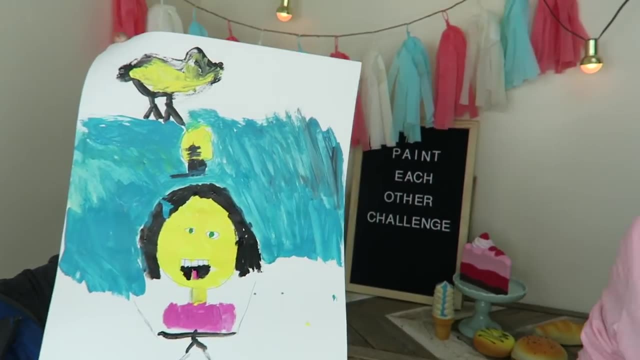 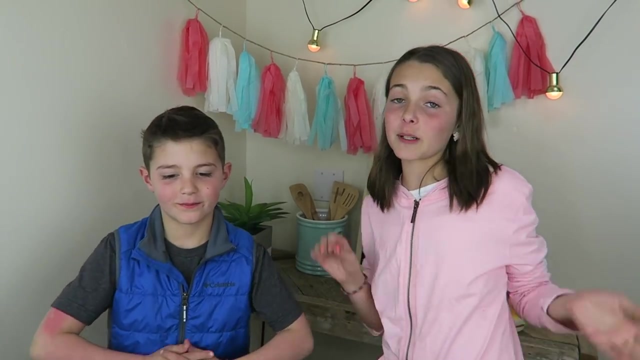 And then there's a watermelon in the grass. I love watermelon. Oh, I like how you added the tongue And my green eyes. That's awesome. Yeah, Yours is really good, Thank you. Okay, guys, let's put them side by side.